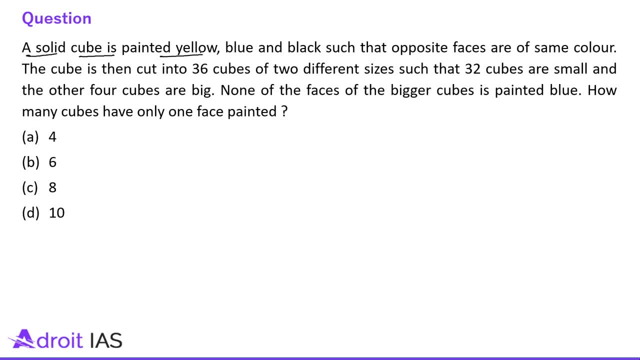 This question says: a solid cube is painted yellow, blue and black such that opposite faces are of same color. The cube is then cut into 36 cubes of two different sizes, such that 32 cubes are small and other 4 cubes are big. 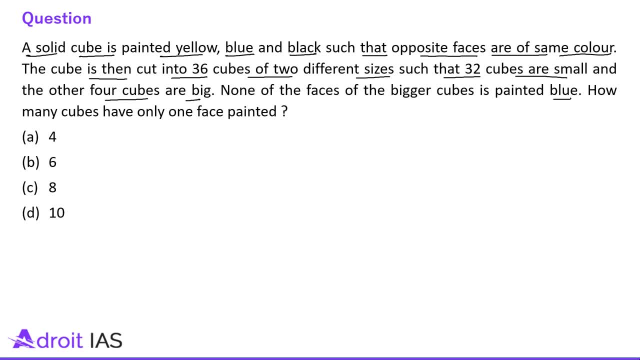 None of the faces of the bigger cube is painted blue. So how many cubes have only one face painted Friends? it is a very good question, And to solve this question a very good imagination skill is required. Why? Because here the cutting pattern is not usual. 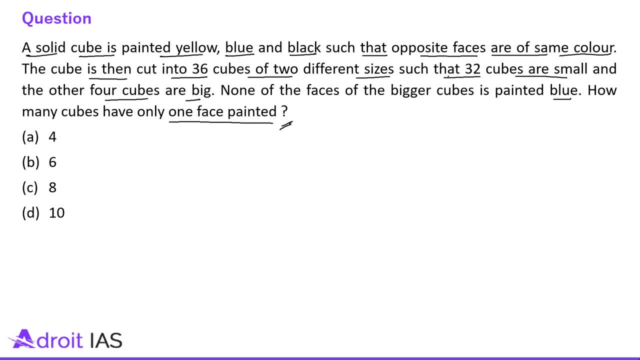 It is slight different than the usual pattern because all the sizes, all the cubes, are not of the same size, right? 32 cubes are small and 4 cubes are big, right? So the cutting pattern will be slight different. So I am showing you the cutting pattern. 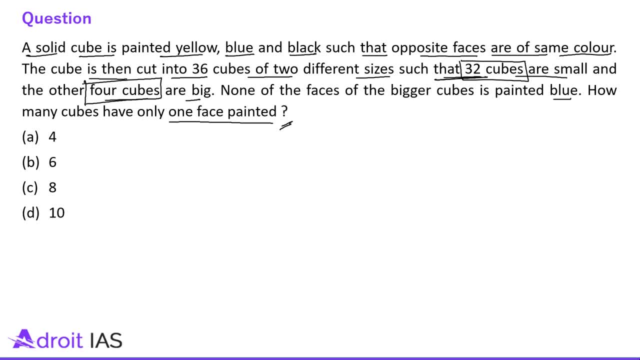 Please try to observe, Observe it carefully. right, This is the cube and this is the cutting pattern. right Here, in the top surface, in the top face, we have 16 cubes, 16 small cubes right And in the bottom face we also have 16 small cubes. fine, 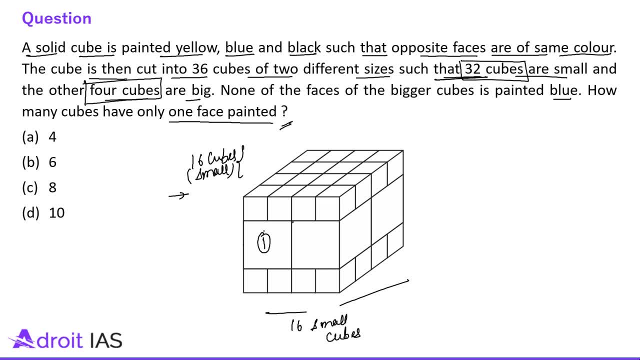 And one big cube is this. another big cube, I mean, one big cube will be like this: Right. Another big cube is this. This. Another big cube is this: Okay, This is number 2,. right, And another big cube is this. and one more big cube will be at the back right. 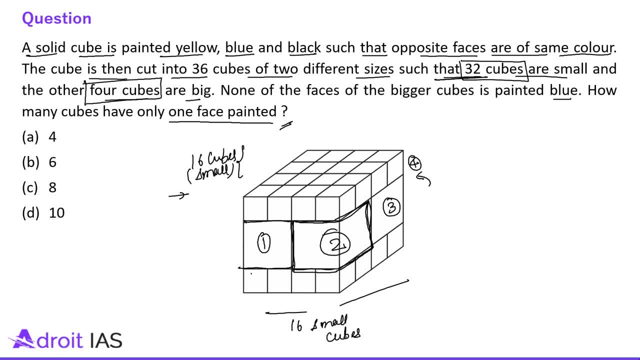 At the back. fine, So we have total 4 big cubes and we have 16 small cubes in the top and 16 small cubes in the bottom right. So total 32 cubes. We have 32 small cubes right. 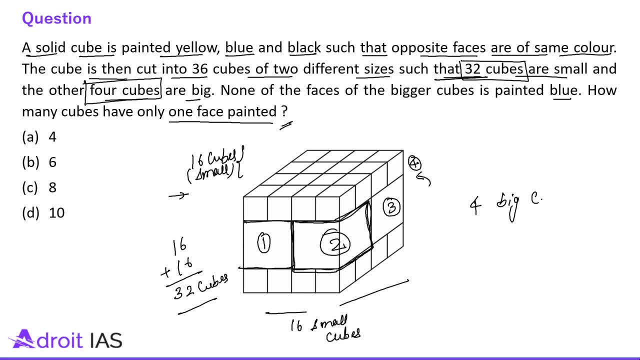 And 4 big cubes, right. So this is the cutting pattern. Okay And everyone. one more thing: question is saying: none of the faces of the bigger cube is painted blue. I repeat: none of the faces of the bigger cube is painted blue. 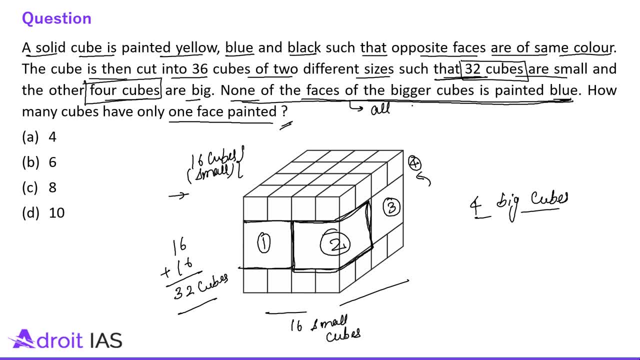 It means what It means. all the, all the small cubes Have been cut from blue face, right? So it means what It means: this top face will be blue, and if top is blue, then bottom will also be blue, because the same color are of opposite faces, right? 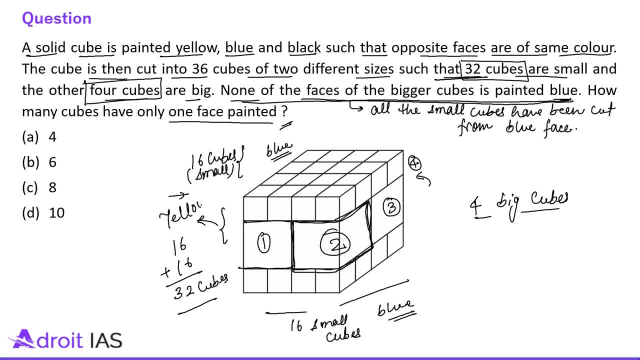 So let's say this is yellow, Okay, And this is, let's say this, this face, this side face. let's say this is black, right, Though now it does not matter because we, we almost have cracked the question, so the color does not matter now, but anyways, we need to find the color also, fine. 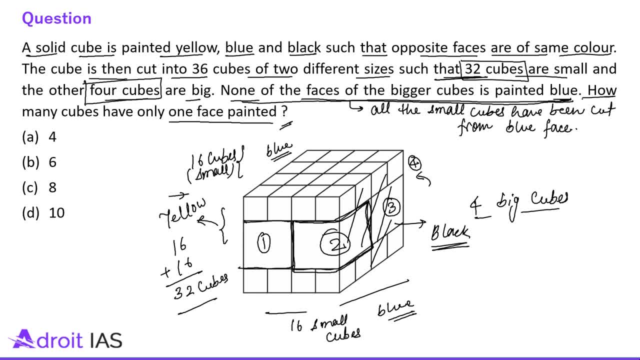 Anyways, let's talk about the question. Question says: how many cubes have only one face painted? Question says: how many cubes have only one face painted right? No, friends, If we talk about the corner one right, The cornered cube. 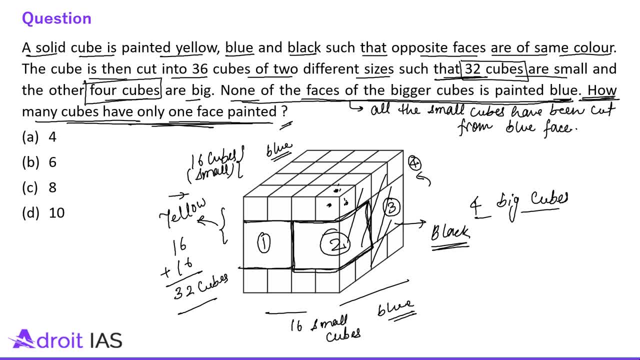 This: this cube is like situated in the corner, So this will have three face painted right, And this cube is on the edge. This will have three, two face painted fine. This will also have two face painted. This will also have two face painted fine. 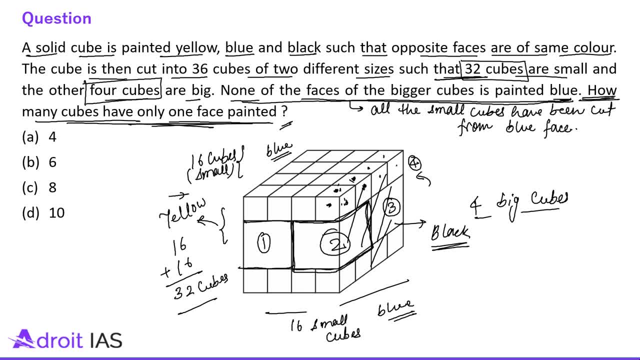 So we will not take into consideration the cubes which we are situated in the corner and the cubes which we are, which are situated in the faces- Sorry, edges right, So edge and the corner. These cubes won't be taken into consideration, right. 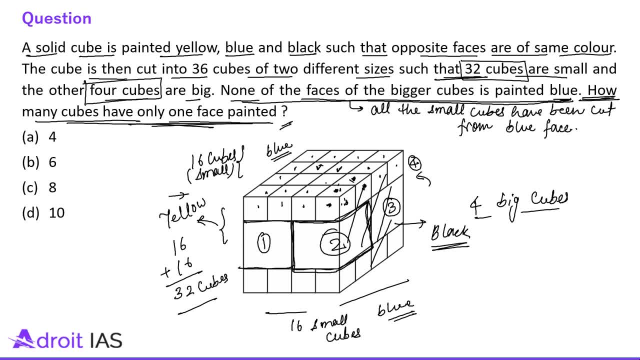 Now the center cube. This, this: These four cubes will have only one face painted right. Hope you must be getting it right. These four faces will have only one face painted right. So four face at the bottom, sorry, four face at the top. 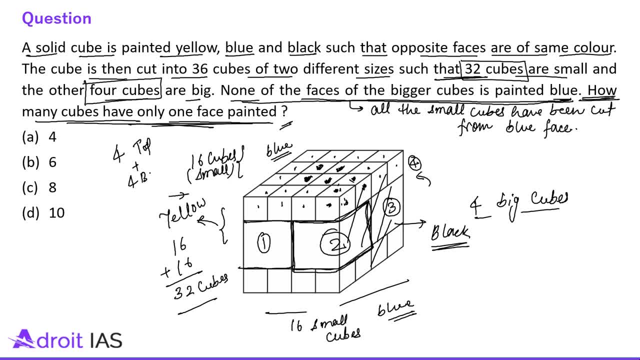 And four face at the bottom And four face at the top And four face at the bottom, will have only one face painted. It means eight total cubes will have only one face painted. fine, The correct answer is three.